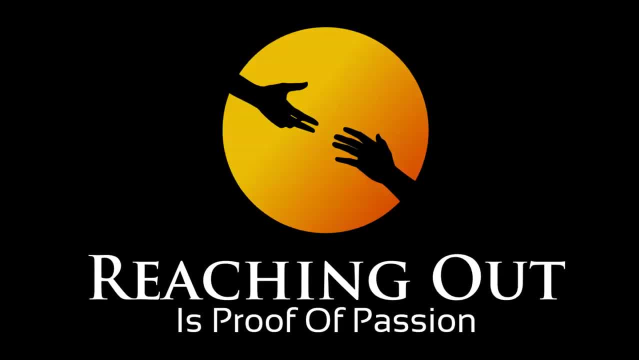 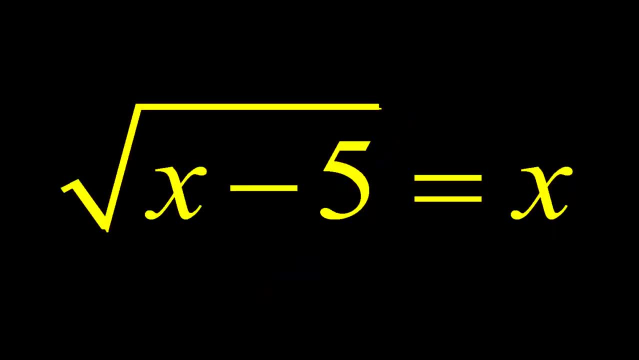 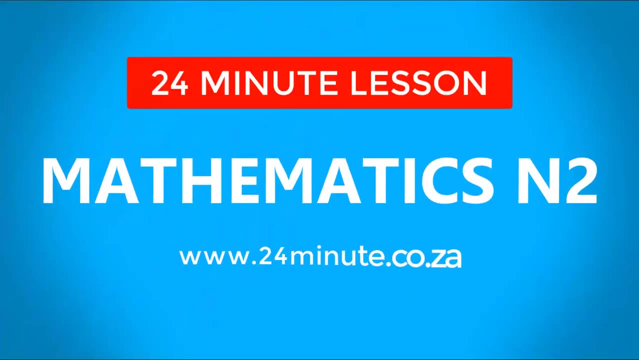 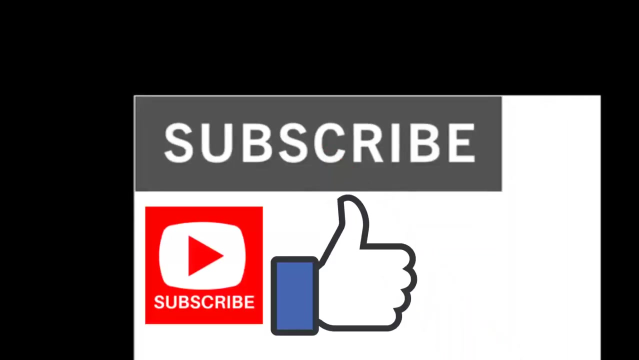 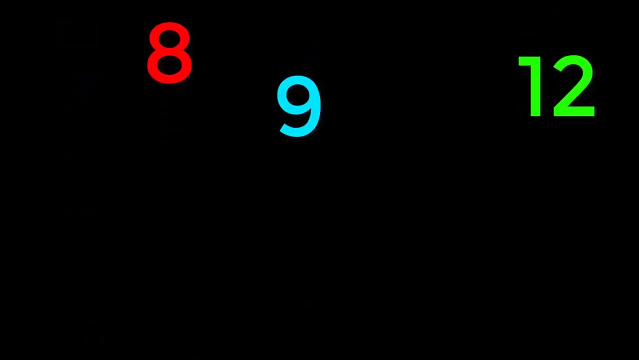 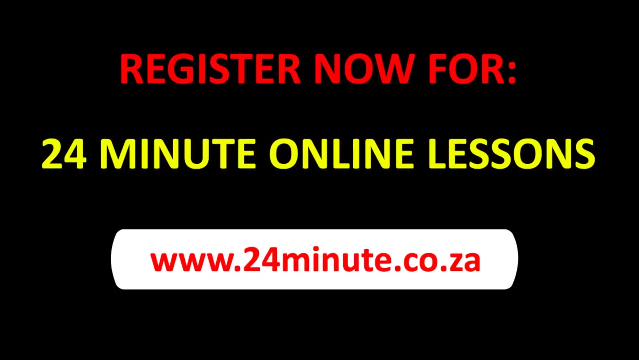 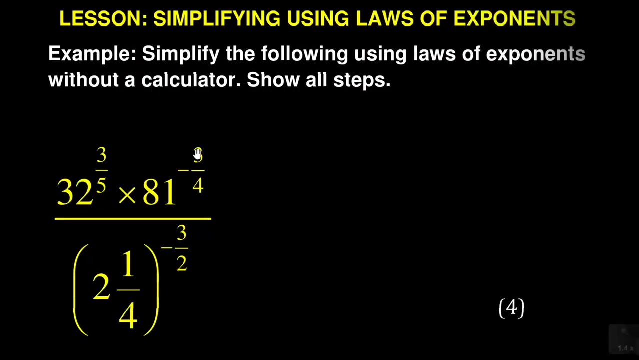 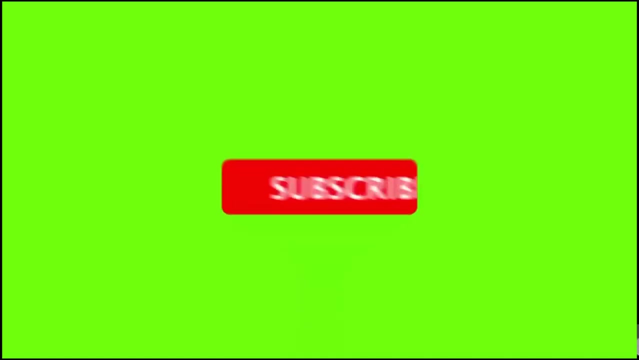 The video is not a video in which you can see the text. The video is not a video in which you can see the text. hello again, our most valid student. my name is confident. welcome to our revision session of mathematics n2. i say it's n2 because i took this from a mathematics n2, but i also encourage. 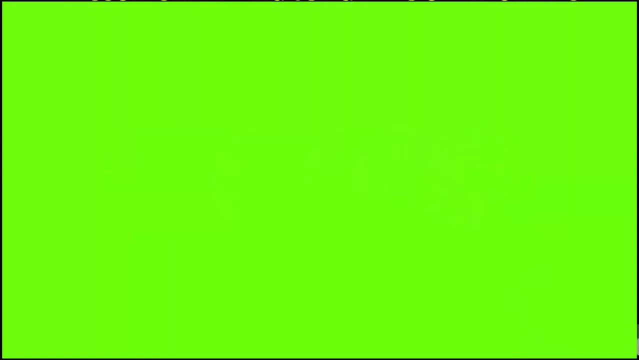 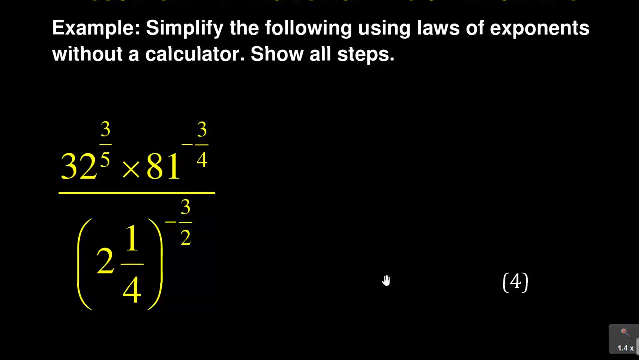 you if you're doing your grade 9, grade 10? this is very important because you can face such questions now. this question was for max, as i say specifically for those who are doing their n2. i just says: simplify the following using laws of exponents without a calculator. then say: show all steps. 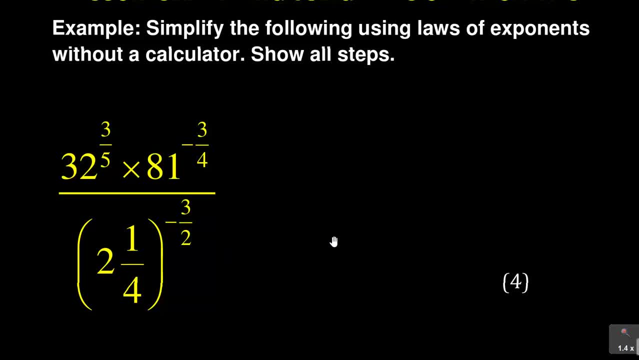 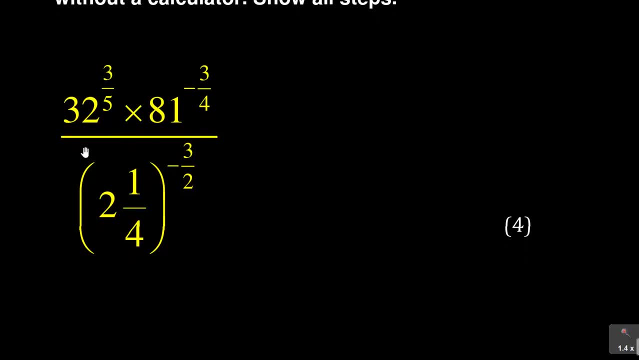 so if you just use a calculator, you won't get any marks and, as i say, guys, it is very important for you to have some idea on how to approach this. now. i will encourage you to subscribe to our channel as well as turn on that notification bell so that you can be notified whenever we bring such uh. 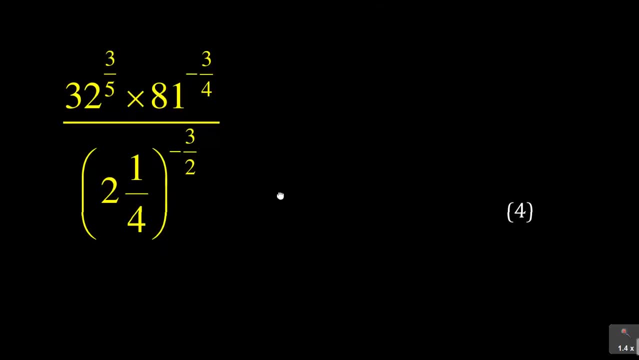 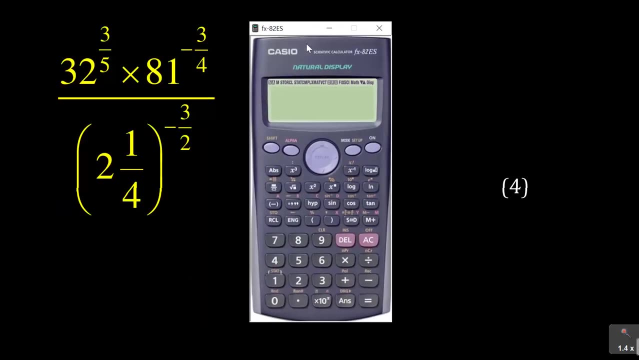 questions to you as you prepare for your final exams. now, how do you solve this? now they say we must not use a calculator. but you know what i do? i just grab a calculator and get my answer. then i work towards the answer. so I've got 32 to the power of 3 over 5, at least I need. 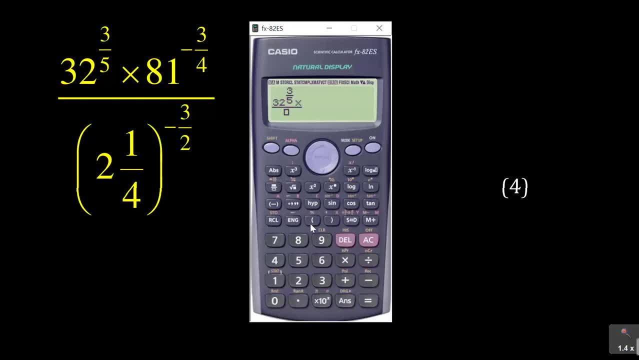 to know where I'm going. so times 81 to the power of negative: 3 over 4 and then over now. this is shift. you do that, say 2 and 1 over 4. this was in brackets. okay, let me just because it's giving me a fun way of the bracket day, so I'll. 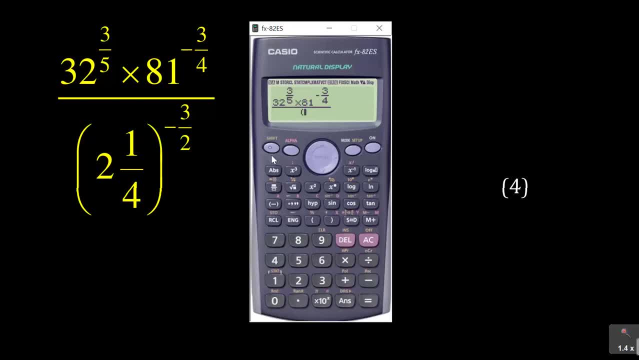 let me do this and then put the bracket and then say shift, have that, that's what I wanted. it's 2 and 1 over 4, like that to the power of negative fraction, 3 over 2. it looks a bit complicated, but you can see that this simplifies to one, so think. 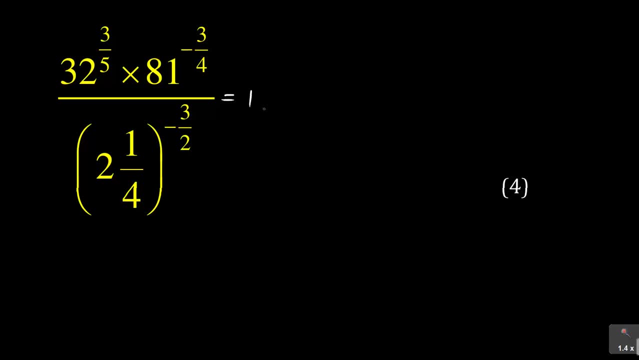 of it as long as you can see that this simplifies to one. so think of it as long it is. i just need to make sure that i get a one out of it now. how do you get one? as i said, use that calculator to advantage so that you can be able to see how you simplify that. now let us use. 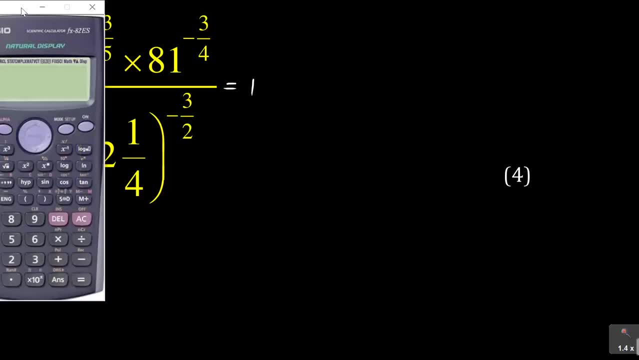 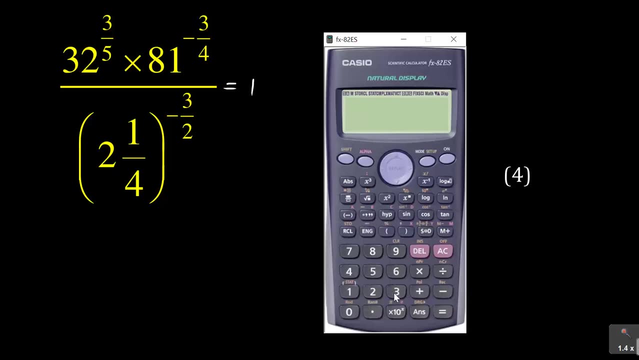 again our calculator to use here. check out: the examiners always give you these numbers intentionally, so they don't just give you numbers which don't make sense. for example, look at 32. 32 is 2 to the power of 5. you see that is 32. 8. 1 is 2 to the power of 3 to the power of 4. 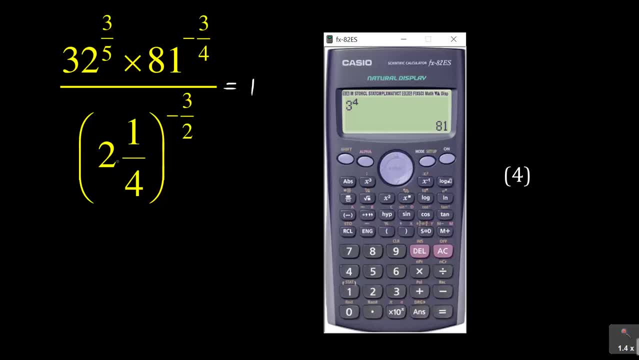 so 3 to the power 4. you see i get 81 now. uh, 2 and 1 over 4. if i say 2 and 1 over 4, it gives me 9 over 4, and 9 over 4 is 3 squared over 2 squared. 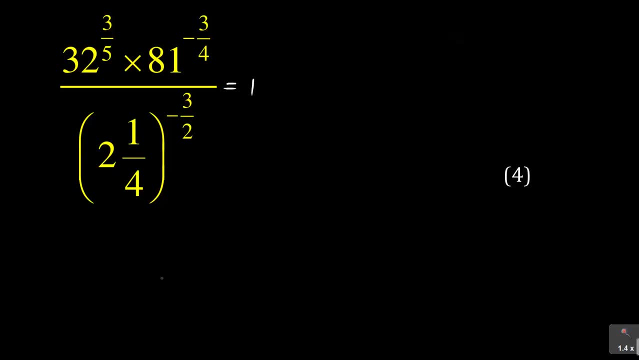 so everything that i'm given here is intentional in a way. so that's what i um these guys do. they always give you something intentionally, so they don't just give you something at random. so we say: 32 is 2 to the power of 5 and then 3 over 5. you see that times 8, 1 is 3 to the power of. 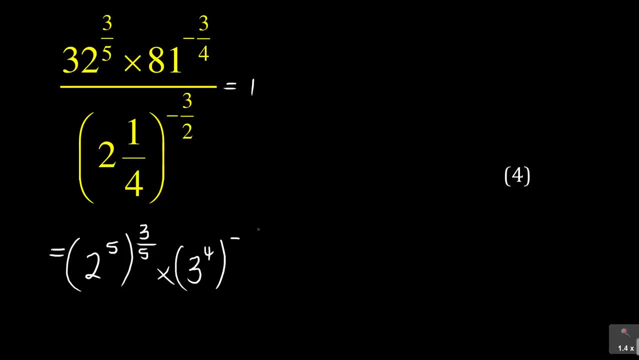 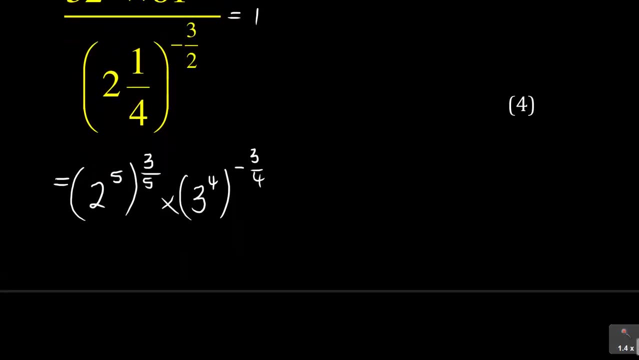 4 again is minus 3 over 4 and then over, as you said this, 2 and 1 over 4. it's 9 over 4. to the power negative: 3 over 2. if you continue simplifying that you're going to have, in this case, equal to, you are multiplying, remember. 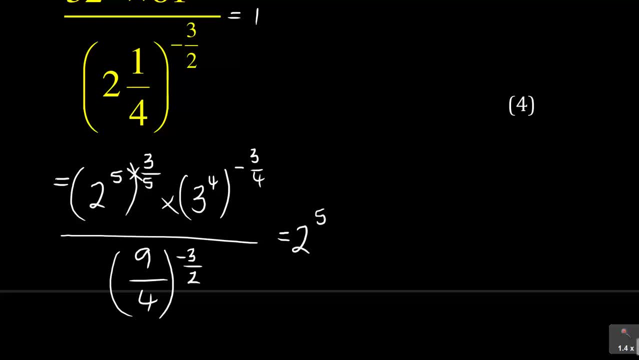 the exponent is actually multiplying 2 to the, The power of 5 times 3 over 5.. This is 5 over 1 times 3 to the exponent of 4 times 3 over 4.. But there was a negative, remember. 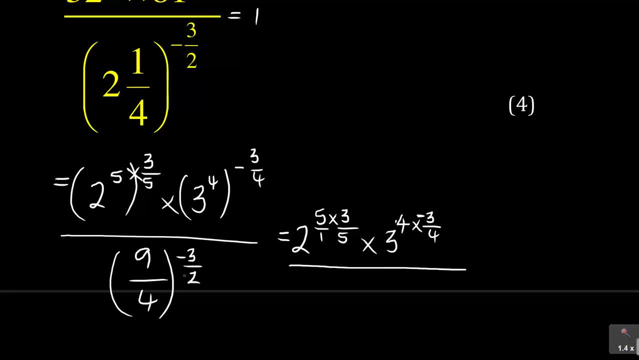 I must not forget that. And then, over Now, this 9 is 3 squared times. okay, let me do this. So it will be 3 squared times negative, 3 over 2.. This is over 1.. These are exponents. 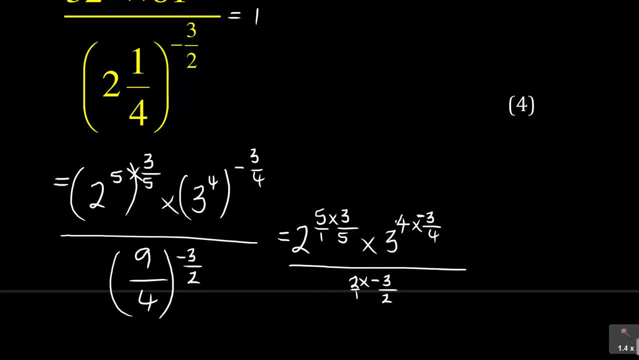 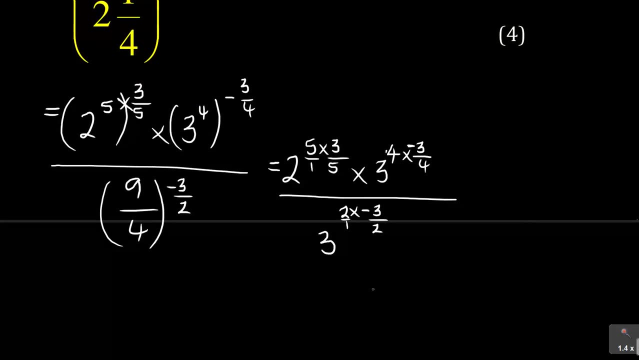 I know I wrote like it's a number now, So let me make this 3 bigger so that it becomes a power there. It's now a bit far, So this is 3.. And then this is over, because this power is affecting 9 and it is affecting 4.. 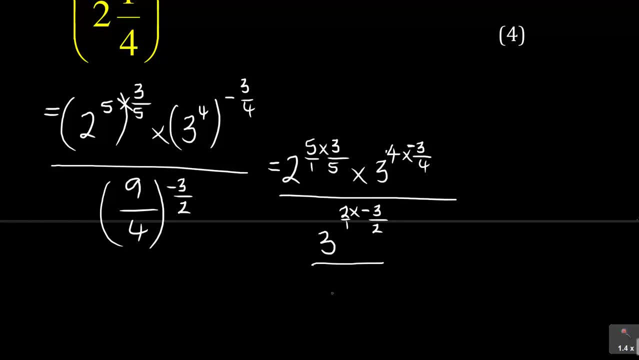 So that's why I'm distributing it already. And 4 is 2 squared times negative 3 over 2.. So you see how this was actually going. Then you can cancel out Things simpler. That 5 cancels, You are left with 2 to the power of 3.. 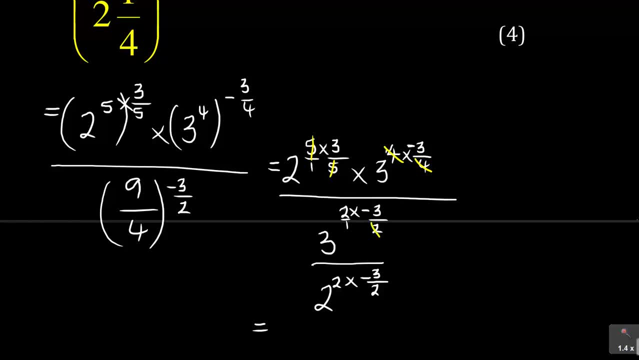 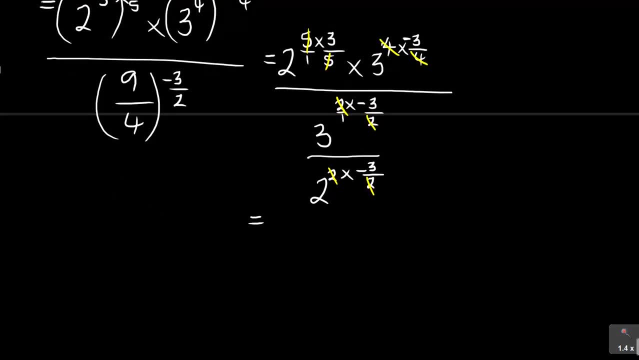 The 4 cancels, And here the 2 cancels, And here the 2 cancels. So you see what you are left with. You'll be left, in this case, with 2 to the power of 3 times 3 to the power of negative 3.. 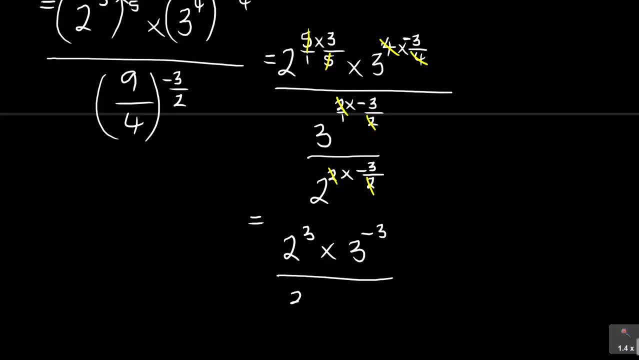 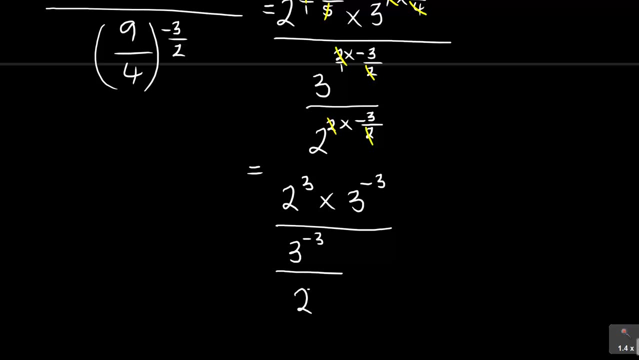 Are you seeing that? All over, 3 to the power of negative 3.. And then over, In this case, it becomes 2 to the power of negative 3.. Are you seeing that, Which is equal to? In this case, if you continue with it, it is equal to. 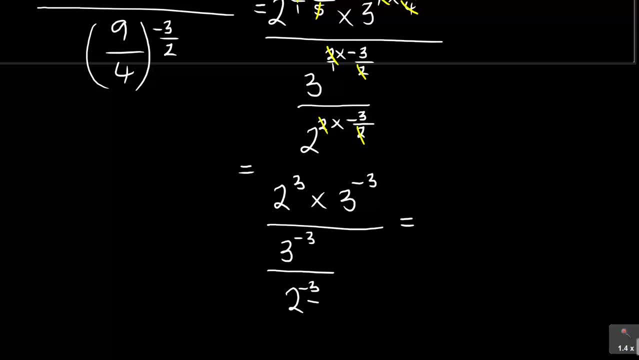 Now it's up to me how I want to do it, But I can take this to the top using this. I'm going to take the top to the top. the law here, the law I'm using. remember, if I'm given 1 over a to the power negative. 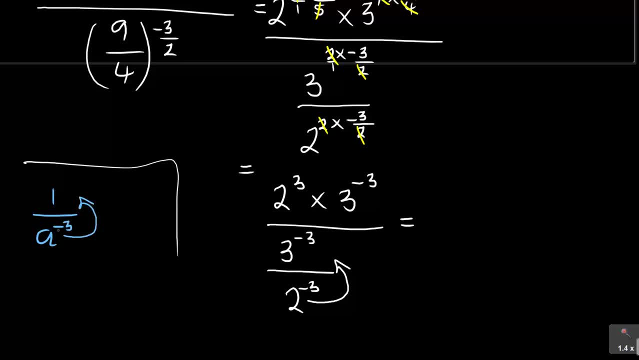 m. if I take it to the top, the negative sign will drop, so it will be equal to 1 to the power m. If I was given 1 over a to the power of 3, it's not m there. I wanted to put an m in. 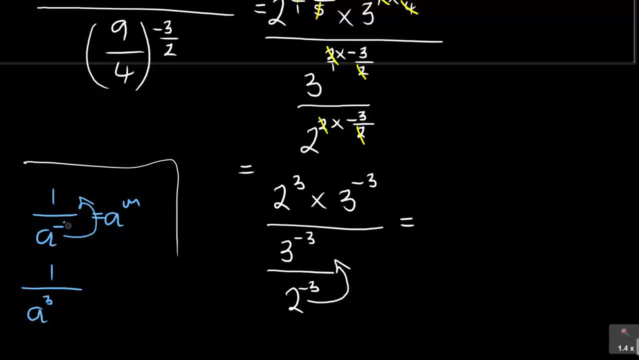 this case here to say it's negative m. So if I've got 1 over negative 3,, if it goes to the top, the negative will drop to become 1 over a to the power of 3, using the same law. So here, if I'm given 2 to the power negative 3, if I take it to the top it will become 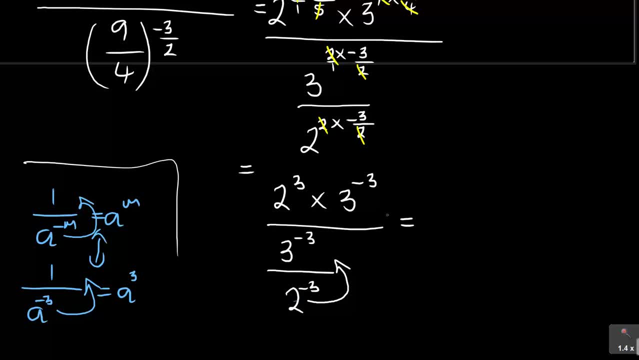 2 to the power of 3.. Times 3 to the power of negative, 3 over 3 to the power of negative, 3. times 2 to the power negative 3 will become positive. 2 to the power of 3.. And if you do that, 3 to the power of that. this cancels, this cancels, that cancels. 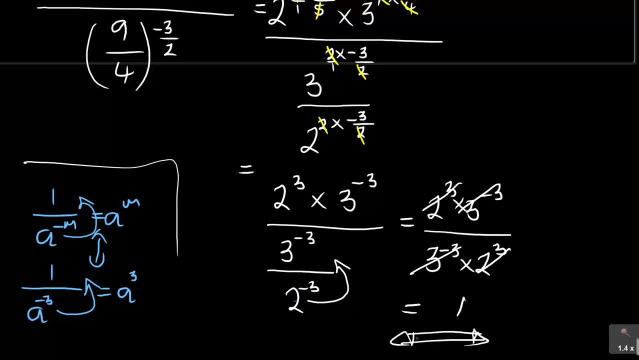 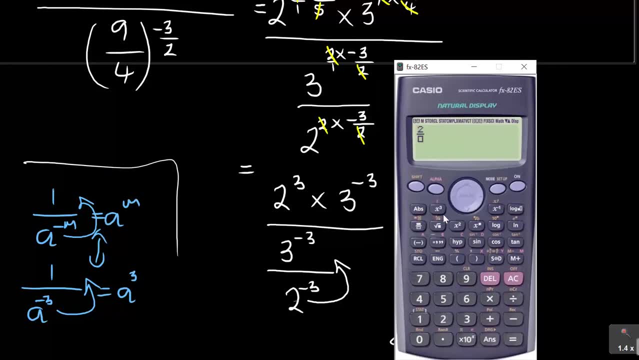 the answer gives us a 1, just like we got it in the previous case. You can even test it with a calculator at this stage here to say you've got 2 to the power of 3 times 3 to the power of negative 3, and then over put a fraction, again 3 to 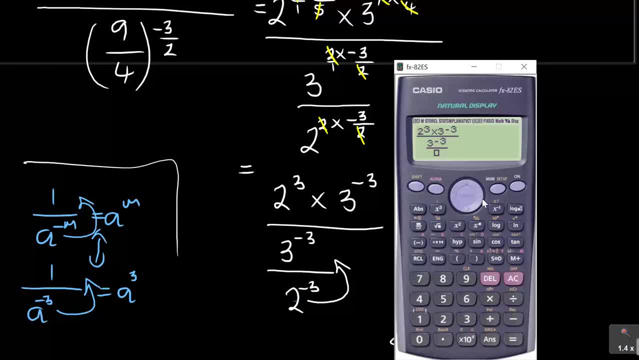 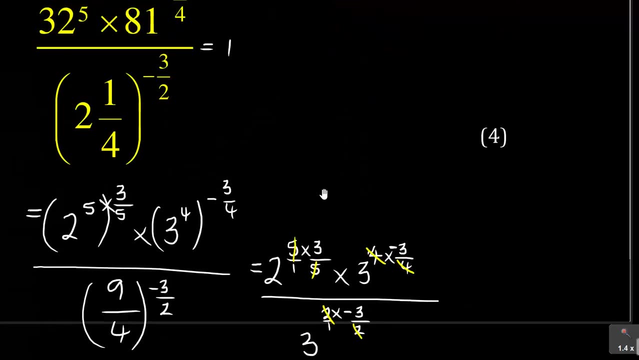 the power of negative 3 over 2 to the power of negative 3.. If you do this, you can see that it still gives us a 1, which further simplifies the way I did. Now remember this 1 is what we got here. 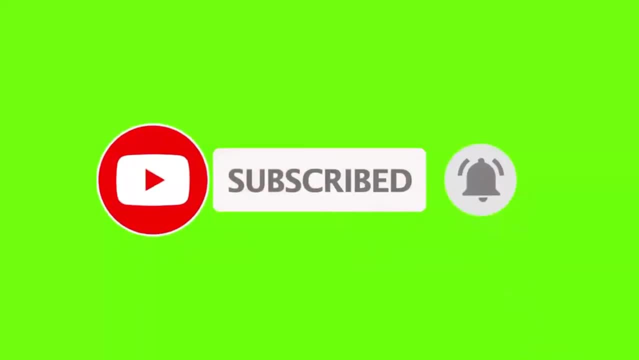 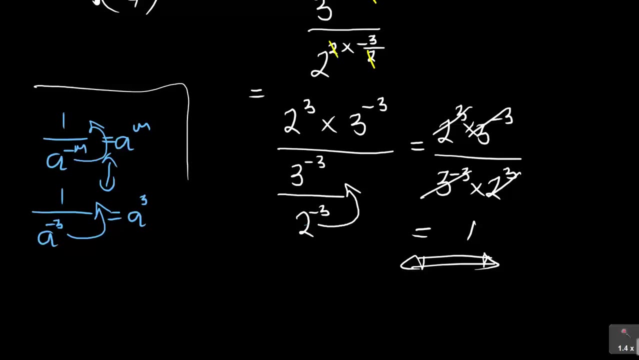 Okay, So it means our simplification is correct. Now, guys, this is what I wanted to bring to you. I hope this was of benefit to you. Now remember to subscribe to our channel so that you can be benefiting as we give these tutorials, so that you can prepare for your final exams.